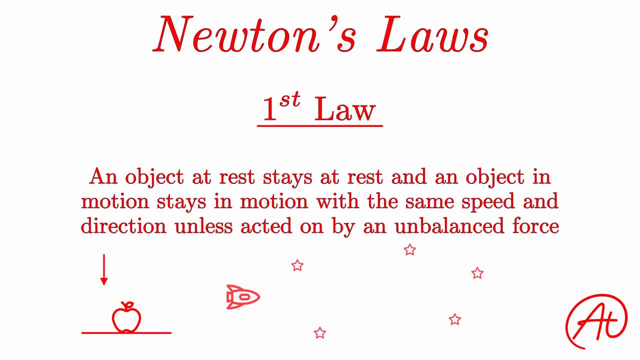 An object in motion stays in motion. If we were to have a rocket moving through space with absolutely no forces acting on it, it will keep going at the same speed and in the same direction forever and ever, until some force starts to act on it. 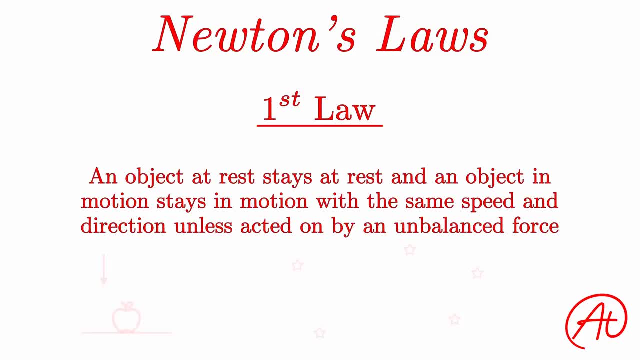 And although this law can be a mouthful, it can be summed up with one word: inertia, which is the tendency for an object at rest to stay at rest and an object in motion to stay in motion. Alright, next we have Newton's second law, which states: an object's acceleration is directly 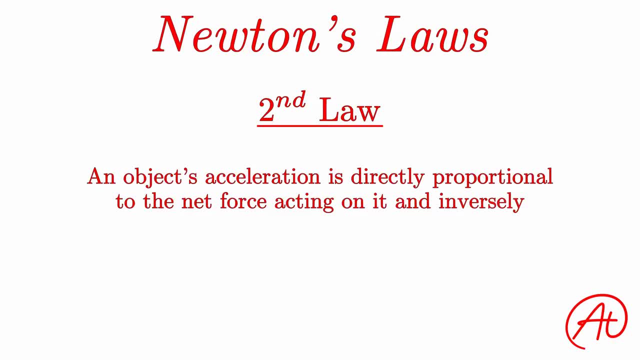 proportional to the net force acting on it and inversely, proportional to the object's mass. So I know this one is also pretty wordy, but these relationships of acceleration, force and mass can be summed up by this equation: Acceleration equals force divided by mass. 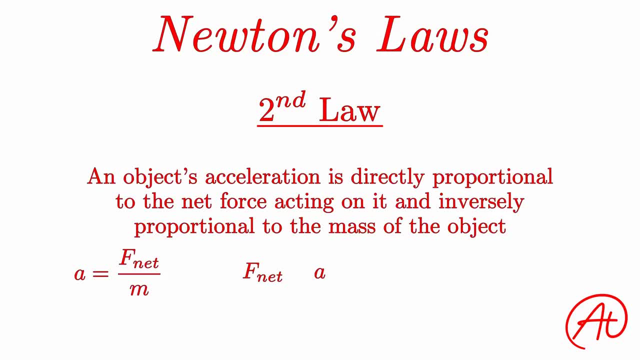 Force and acceleration are directly proportional. So if the net force applied increases, so does the object's acceleration, And if the force decreases, the acceleration also decreases, Which makes sense. If you were to push an object harder, AKA increase the force applied, you would be able. 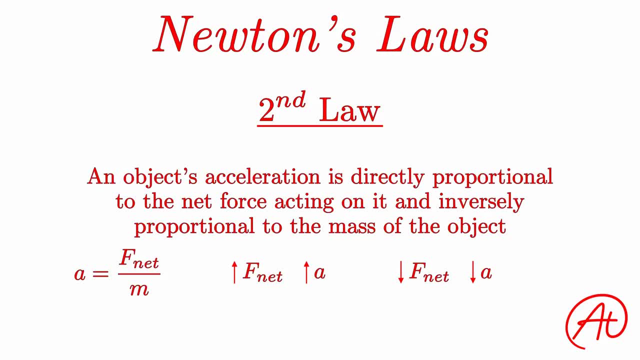 to move the object faster than if you only pushed it lightly. Next, mass and acceleration are inversely proportional. So if the mass of an object increases, the acceleration of an object increases of it would decrease for a certain applied force. Then if the mass decreases, the acceleration would. 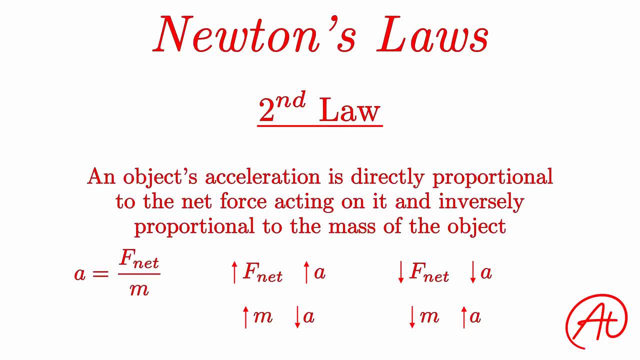 increase, And this kind of makes sense too. If you tried pushing a massive boulder, you wouldn't be able to move it as fast as you would be if it were only a small rock. And if you don't recognize this equation now of acceleration equals force divided by mass, you may recognize it in a more commonly. 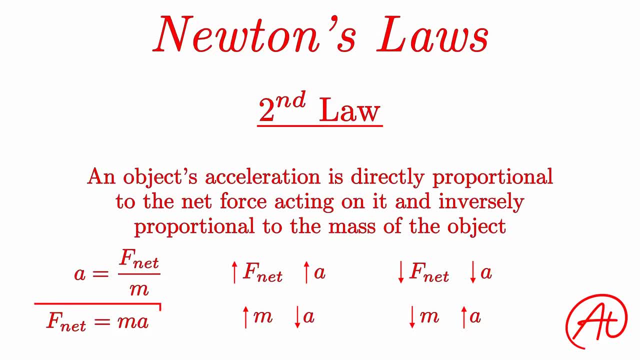 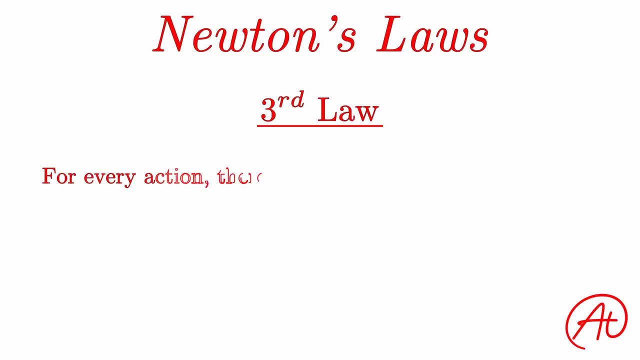 used form of the almighty equation: F equals ma. And finally we have Newton's third law. This one says that for any action there is an equal and opposite reaction. Essentially, what this means is that any action comes in the form of a pair of equal and opposite forces.